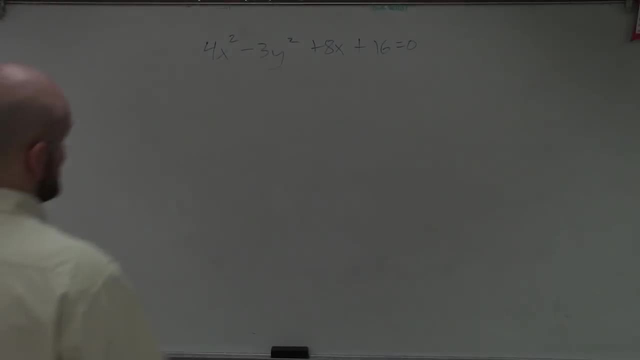 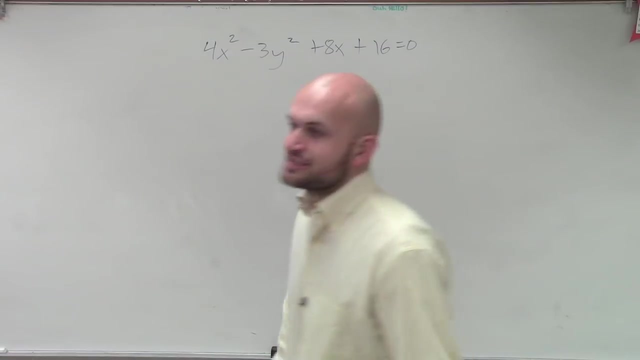 So, ladies and gentlemen, we have an equation, We want to write it into our standard form, and then we want to plot the asymptotes and make a little sketch of the graph. How does that sound? That sounds good, Okay. so the first thing is again, if you know our definition. 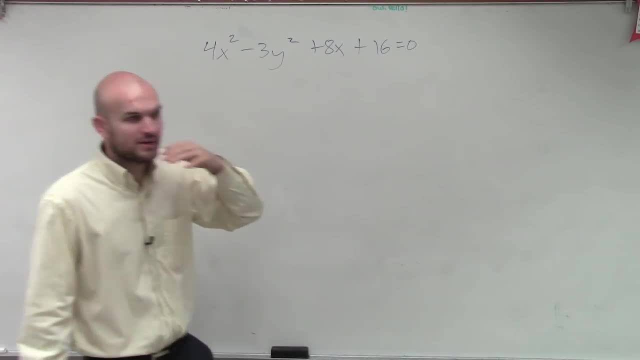 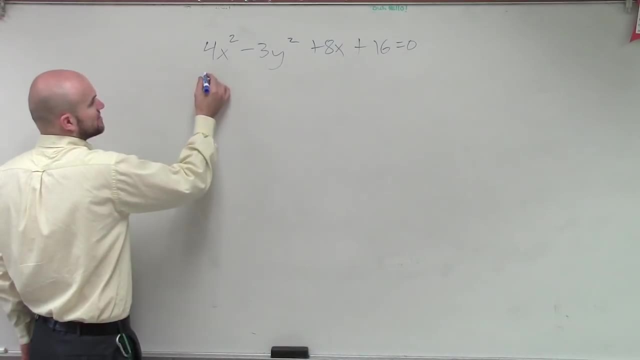 of our parabolas. we need to first, you know, before we can even determine if it's going to be horizontal or vertical, we need to at least be able to see what the graph is going to look like. So the first thing we do is I'm going to combine my 4x squared plus. 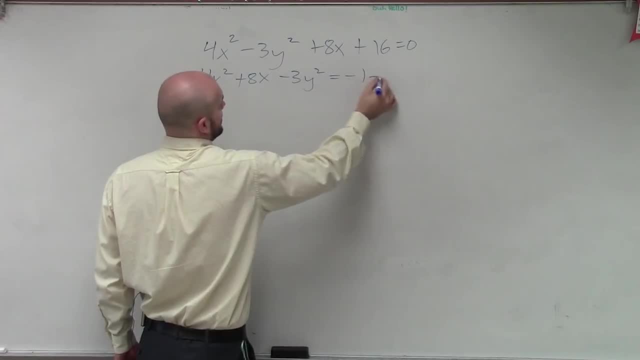 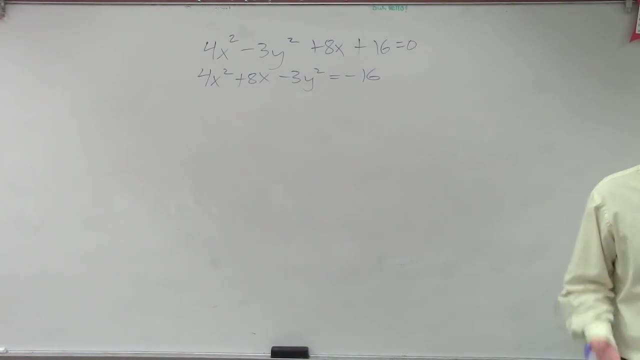 8x minus 3y squared equals a negative 16.. So I put the constant on the other side and I arrange my x's and my y's. And I do that because now I want to make sure that I can combine them, because actually I forgot to go over this. 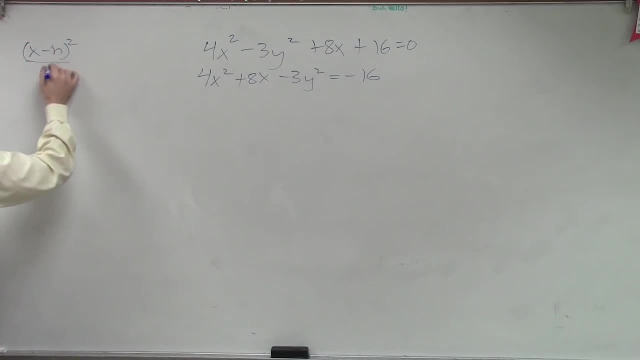 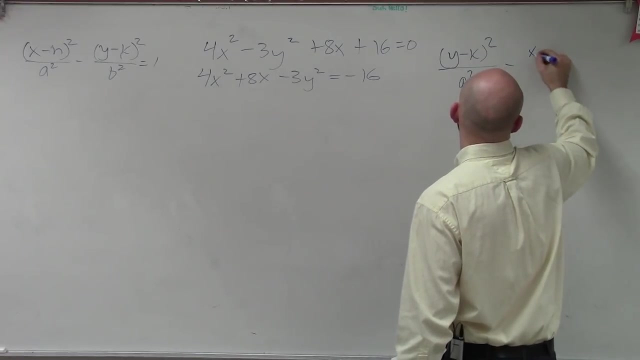 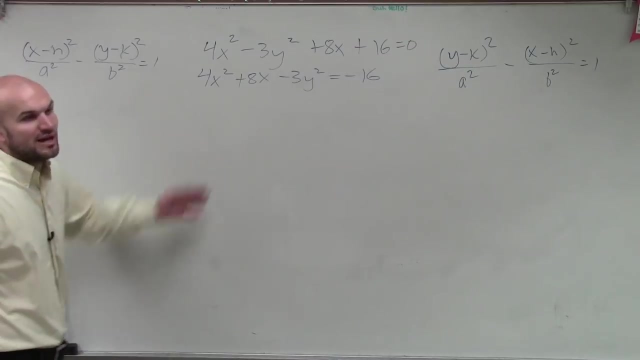 Let's go over the formulas, right, that we're trying to figure out. Okay, this one is x minus I don't know. this one would be y minus k. Okay, so we have our two formulas, And what we need to do is we need to make sure we can write this in that formula, right? 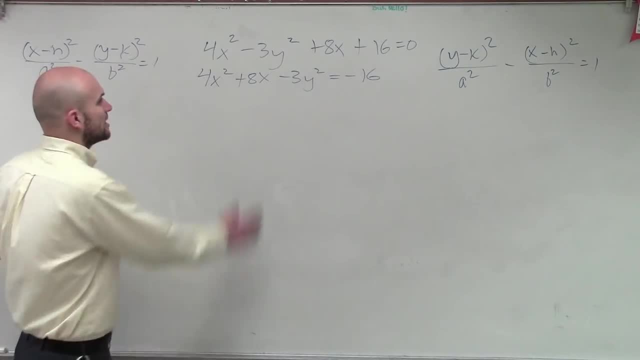 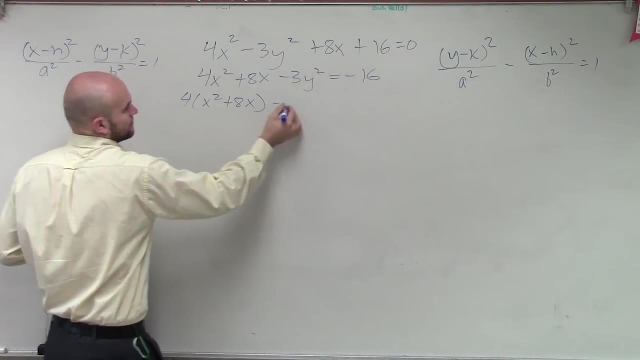 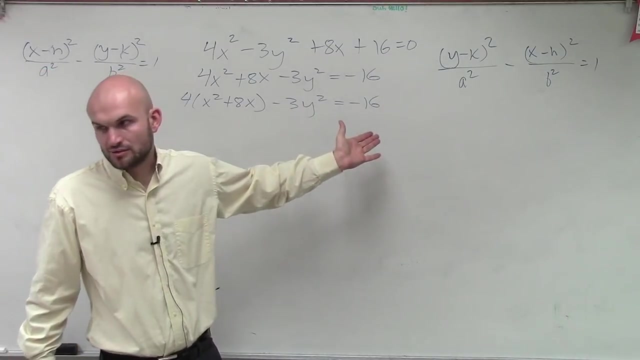 So first thing I need to do is now I'm going to have to complete the square. Before I complete the square with the x, I need to make sure I factor out a 4.. I can't complete the square with my negative 3, but that's fine. That just means that my k is going to be 0, right. 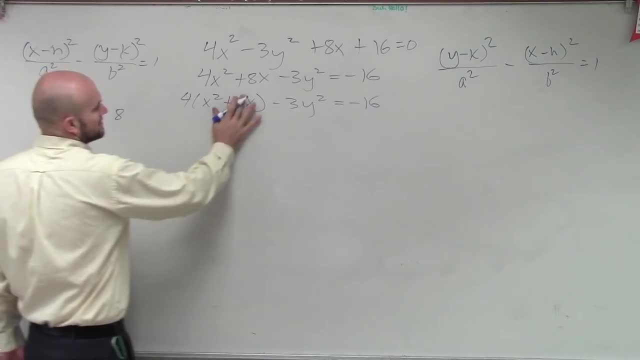 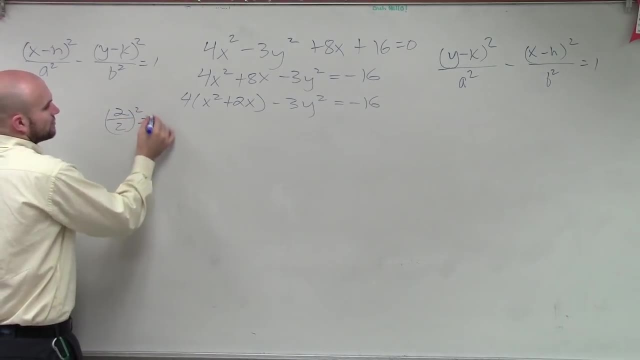 Now I complete the square over here, so I have 8.. Got to factor out a 4,, so that's 2.. So I have 2 divided by 2 squared, which equals 1.. So I have 4 times x squared, plus 2x plus. 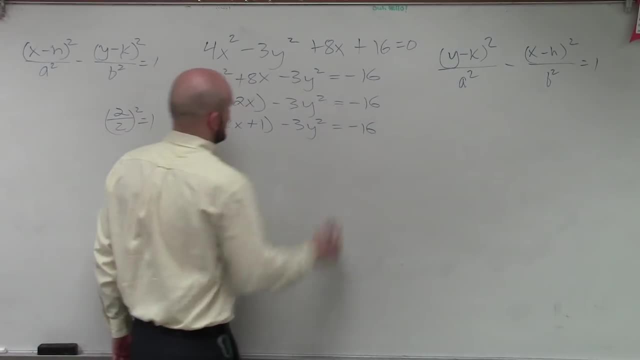 1 minus 3y squared equals negative 16.. However, ladies and gentlemen, notice that I'm not adding a 1, I'm adding a 1 that's being multiplied by a 4, so, therefore, I'm going to have to. 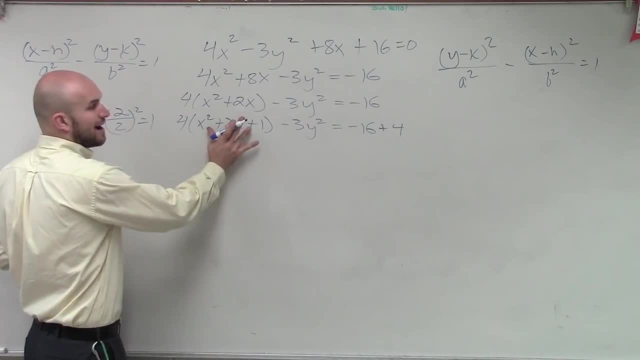 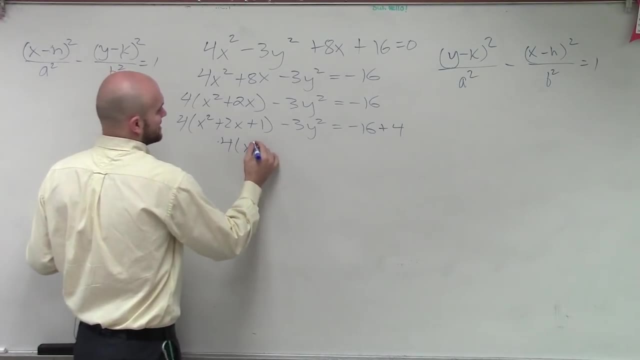 add a 4 over here as well. So therefore now I simplify or I factor this down to a perfect square or binomial square, So it's x plus 1 squared. So I have 2 divided by 2 squared, which equals 1.. So I have 4 times x squared plus 2x plus. 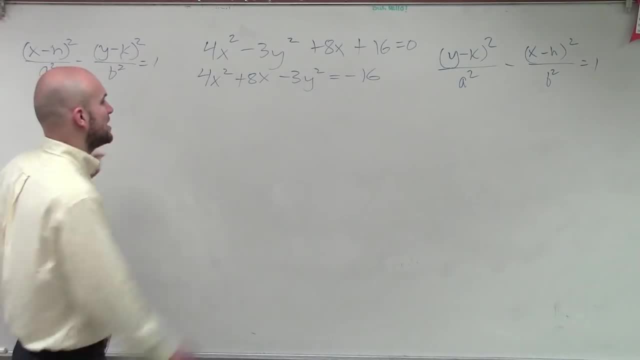 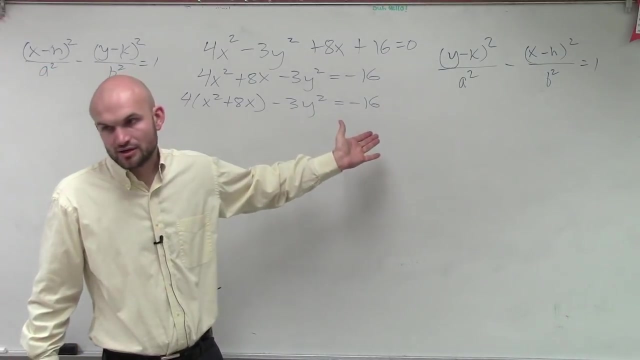 So first thing I need to do is now I'm going to have to complete the square. Before I complete the square with the x, I need to make sure I factor out a 4.. I can't complete the square with my negative 3, but that's fine. That just means that my k is going to be 0, right. 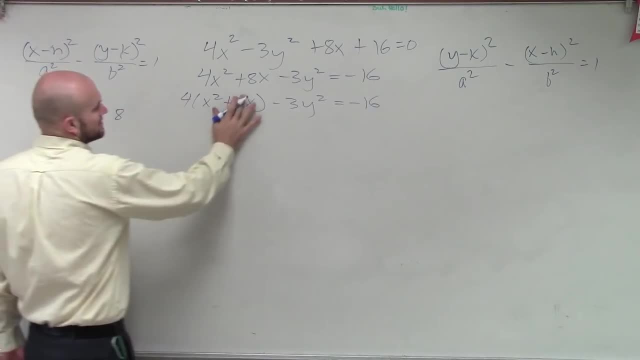 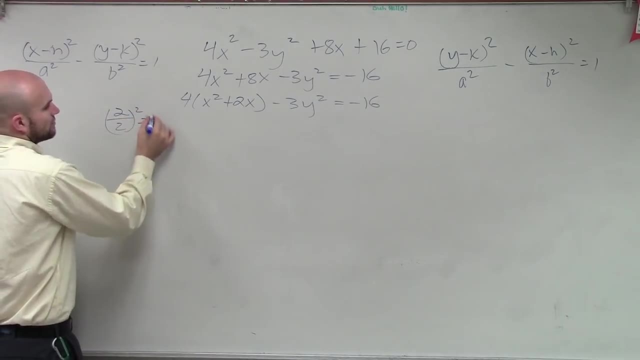 Now I complete the square over here, so I have 8.. Got to factor out a 4,, so that's a 2.. So I have 2 divided by 2 squared, which equals 1.. So I have 4 times x squared, plus 2x plus. 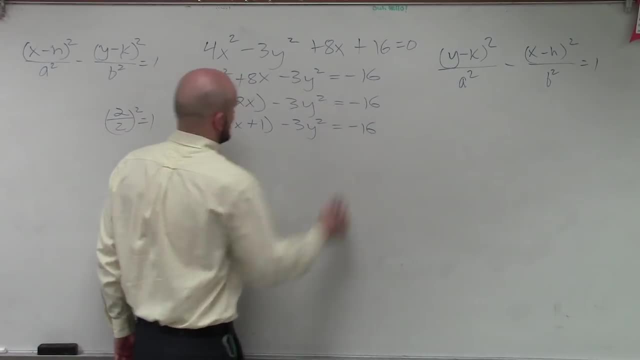 1 minus 3y squared equals negative 16.. However, ladies and gentlemen, notice that I'm not adding a 1, I'm adding a 1 that's being multiplied by a 4, so, therefore, I'm going to have to add a 4 over here as well. 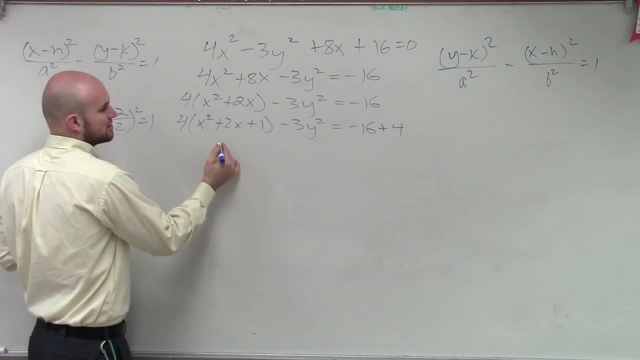 So therefore, now I simplify, or I factor this down to a perfect square or binomial square. So it's x plus 1. So I'm going to have to add a 4 over here as well. So therefore, now I simplify, or I. 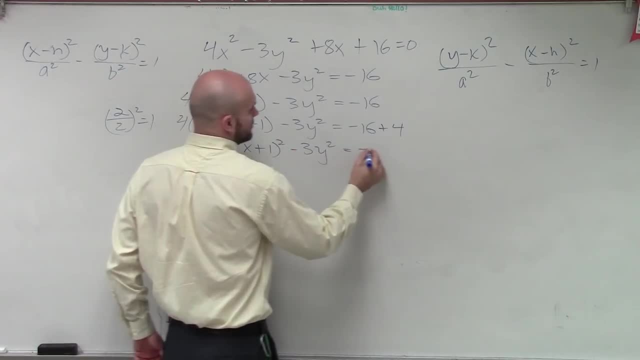 factor this down to a perfect square or binomial square, So it's x plus 1.. So I'm going to have a 6.. So here's the nosso: 0 plus x squared minus 3y squared equals negative 12.. 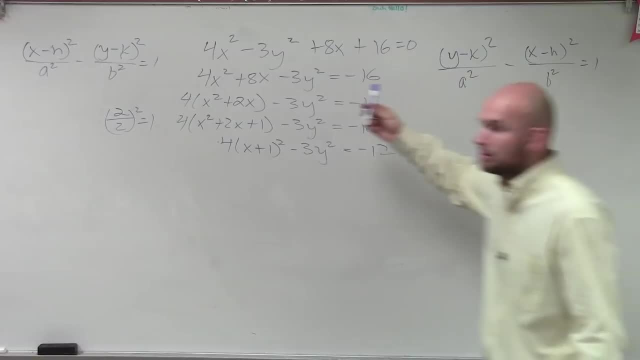 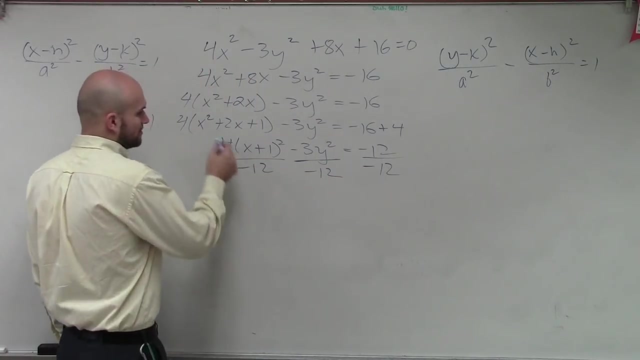 Now again, remember: both of our formulas equal 1, right? Both those formulas equal 1.. So let's divide by negative 12, and we'll do this by both terms. Therefore, by simplifying this, I now have a x squared minus 3.. 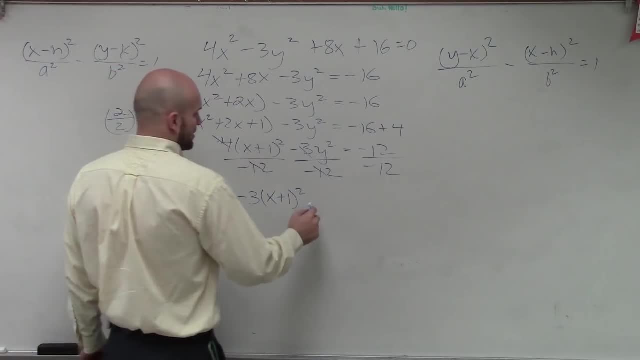 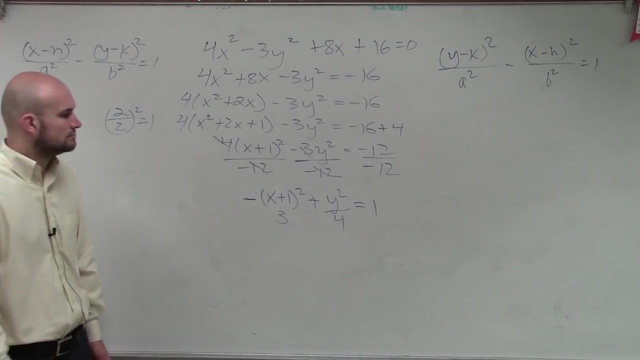 That's equal 1. Remember right times: x plus one squared plus y squared over four. I'm sorry, that's a three on the bottom right. Whoa, did you make the top negative and not the bottom? 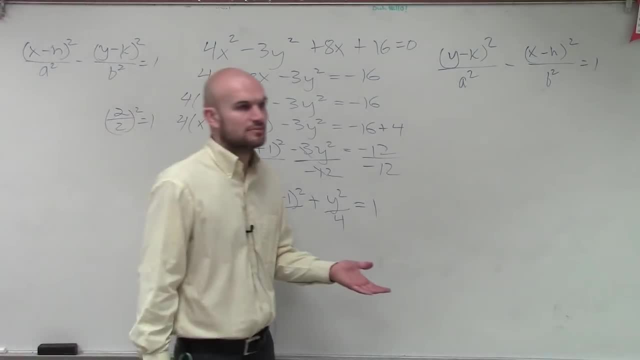 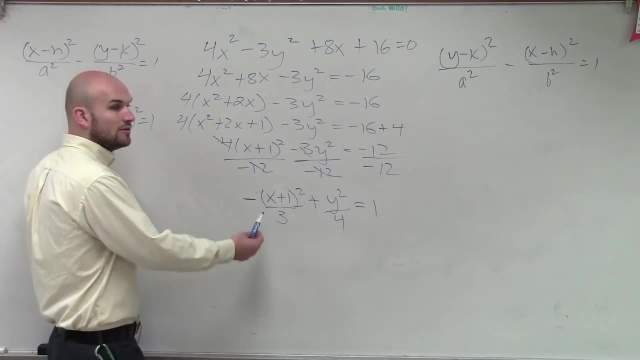 It doesn't matter. Negative four divided by two is the same. Why are you adding? I thought it was multiplying, Because The negative is divided by another negative. that makes it positive, right, True, So now you're right, though. 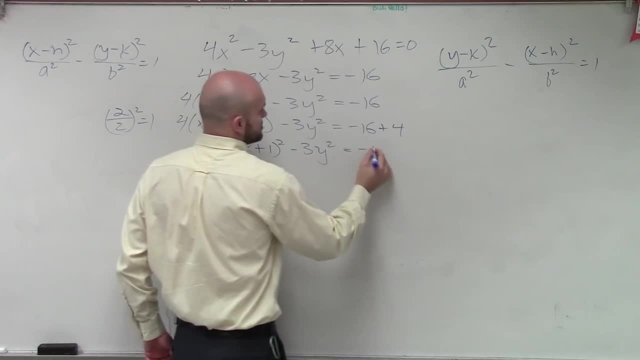 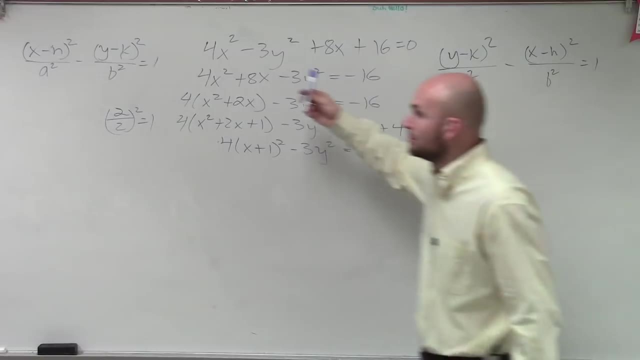 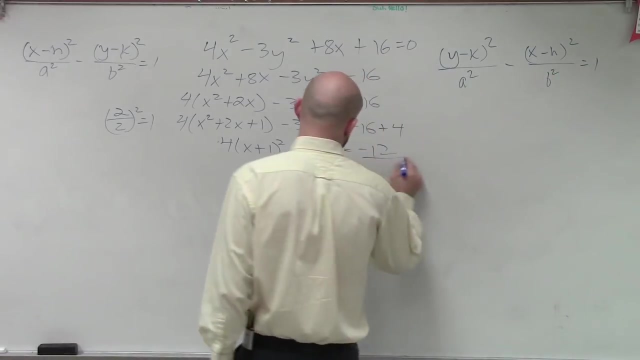 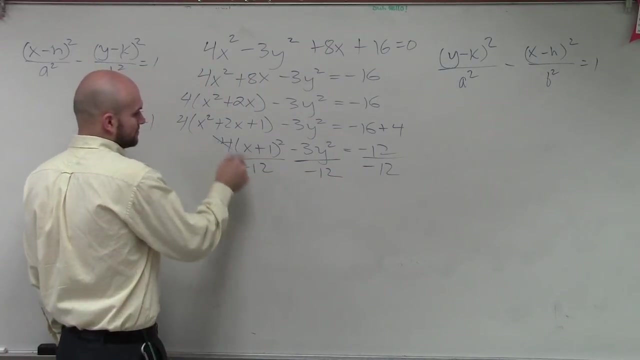 1 squared minus 3y squared equals negative 12.. Now again, remember: both of our formulas equal 1, right? Both of those formulas equal 1.. So let's divide by negative 12, and we'll do this by both terms. Therefore, by simplifying this, I now have a negative 3 times negative. 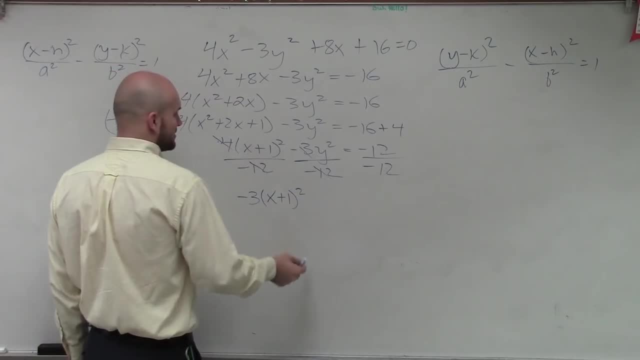 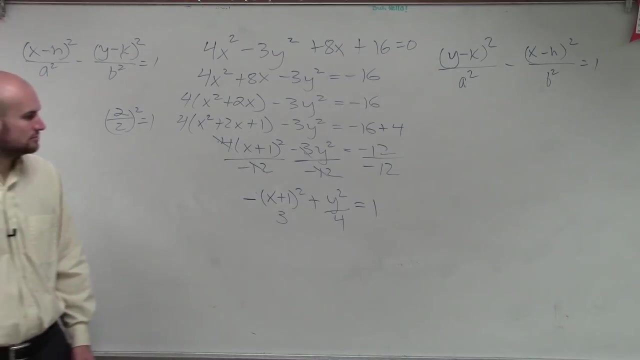 12. So I have 3 times x plus 1 squared plus y squared over 4.. I'm sorry, that's a 3 in the bottom right. Whoa did you make the top negative and not the bottom? It doesn't matter Negative. 4 divided by 2 is the same. 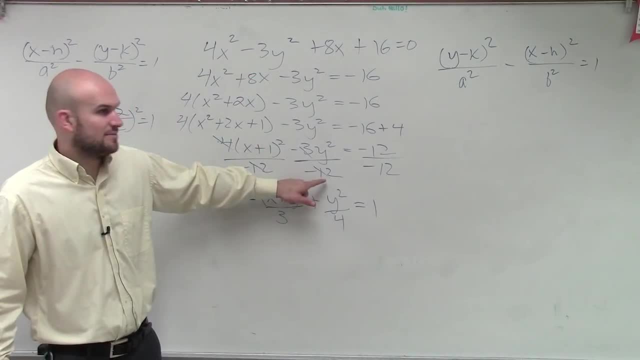 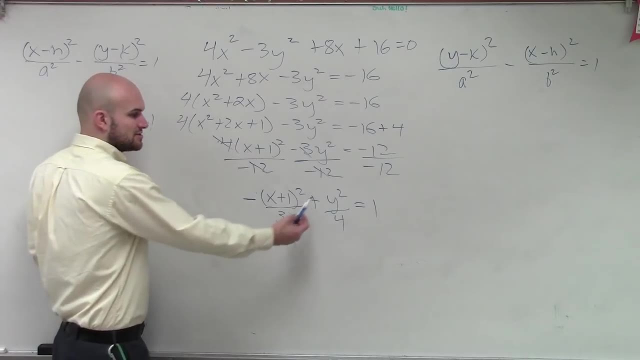 Why are you adding? I thought it was multiplying. The negative is divided by another negative. that makes it positive, right? True? So now you're right, though This needs to be a subtraction problem. So I'm going to subtract your problem, right? So, rather than saying a negative number plus a positive, 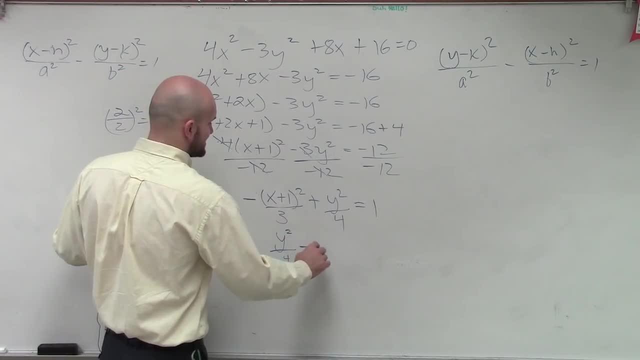 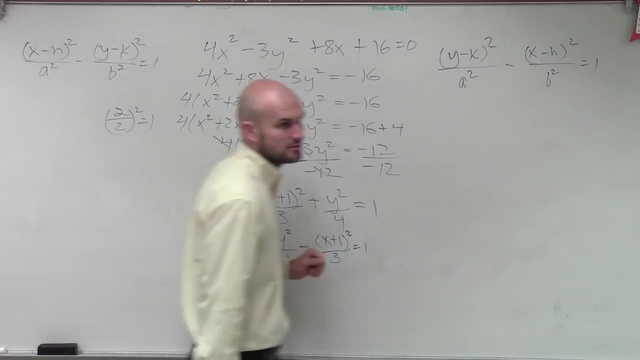 I can rewrite this as: y squared over 4 minus x plus 1, squared over 3, equals 1.. So you're right, You want to write it in that format, because now, when you have it as a subtraction, you know now that a squared equals 4 and b squared equals 3, right? 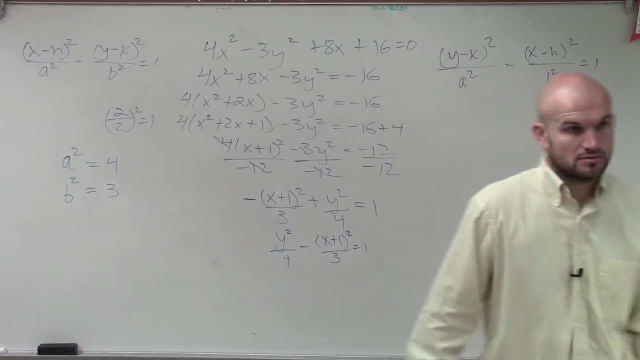 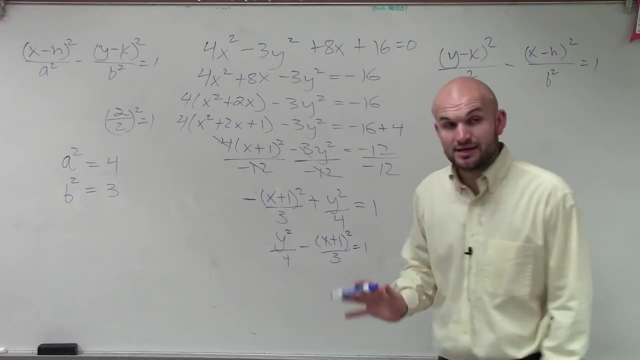 How do you know? I don't know, Because it's always a squared minus b squared. for a hyperbola: A squared minus b squared. No, not necessarily. It's just always in the formula: a squared minus b squared, That's. 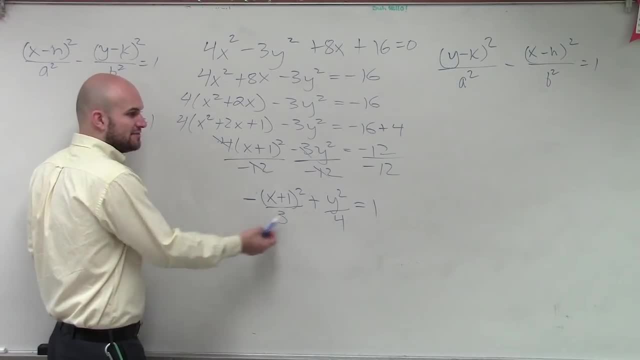 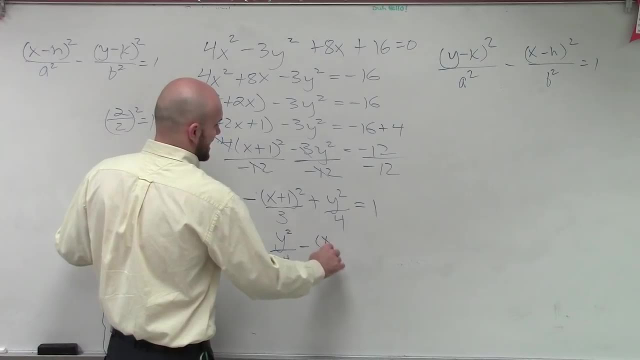 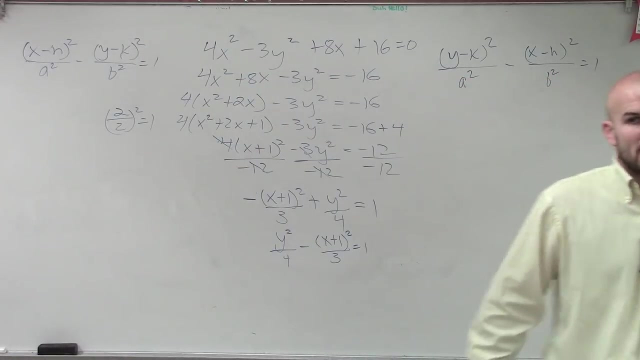 this needs to be a subtraction problem, right? So, rather than saying a negative number plus a positive, I can rewrite this as y squared over four minus x plus one squared over three equals one. So you're right. Right, you want to write it in that format. 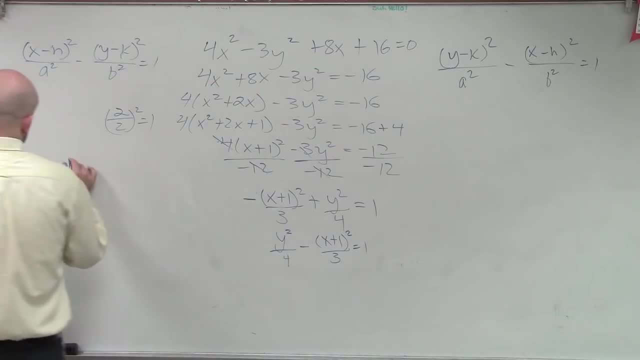 because now, when you have it as a subtraction, you know now that a squared equals four and b squared equals three. right, Because it's always a squared minus b squared. for a hyperbola: A squared minus b squared- huh. 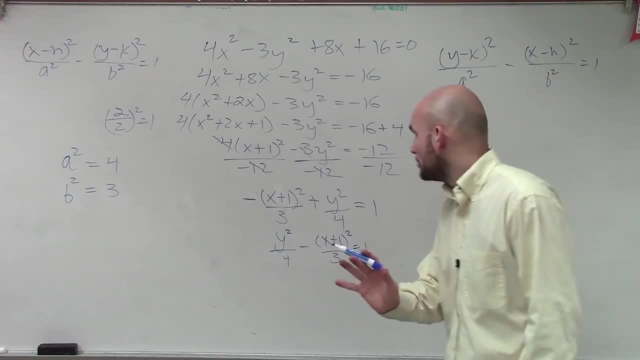 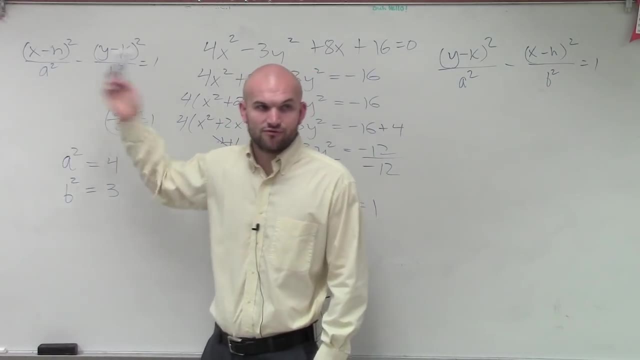 A is always the larger one, right? No, not necessarily. it's just always in the formula a squared minus b squared. that's the formula that we're always going to have in this form. So in hyperbola it's a quantum out of a bigger or a smaller one. 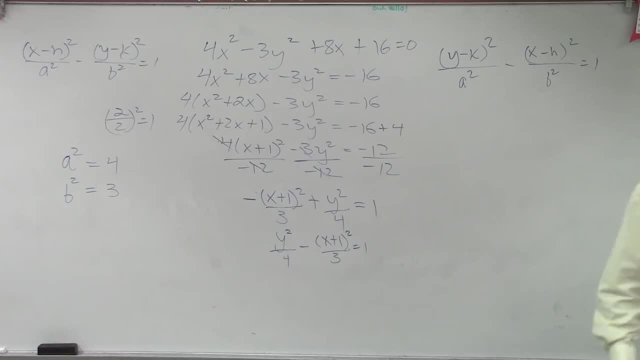 You're not always going to have a larger or a smaller one, But I thought you said that the a squared On your ellipse, on the ellipses. that's the way that you're always going to have it, Okay. So how do you know? when you're subtracting? 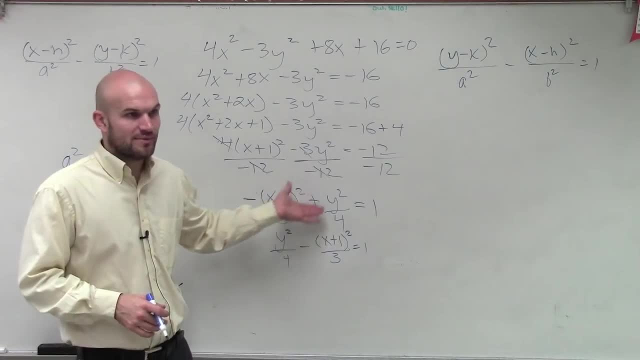 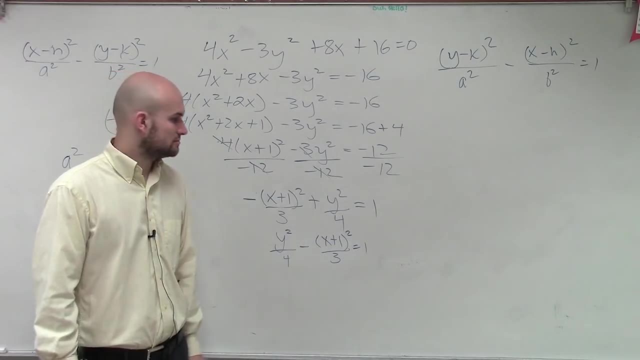 You just write it as your subtraction, one minus the other, and then whatever that is, whatever you subtracted from that's your a minus your b, So it can be related. It can be four minus five. Yeah, that was our last example, right? 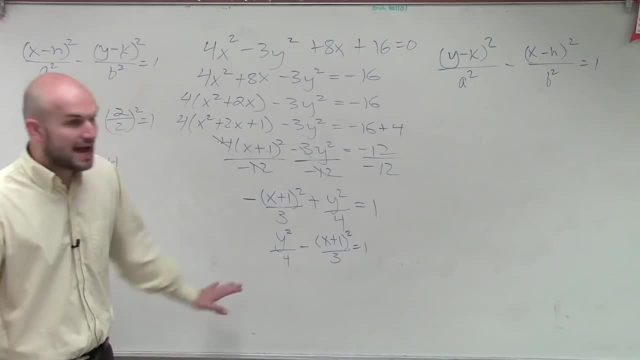 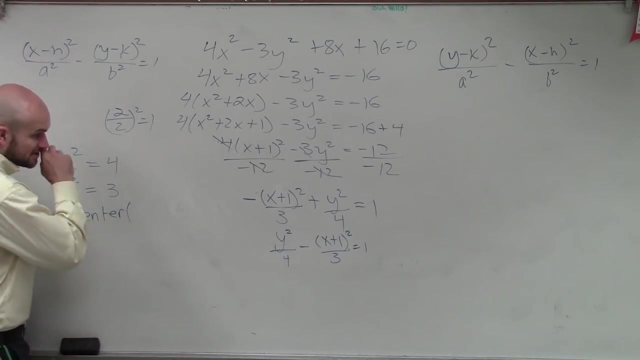 So now let's go and take a look at our h and our k. So if we know our h is now represents, let's just do our center. So now you have your a squared and you have your b squared. So now I can say the center is going to be negative one comma zero. 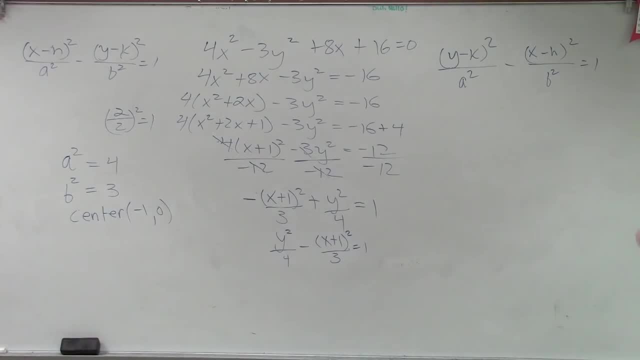 Yes, yes, no, maybe so, okay. So, ladies and gentlemen, if we have our four and our y, if our a squared is under our y, now, this means we're going to have a vertical one right Vertical, So we know our center's at negative one, zero. 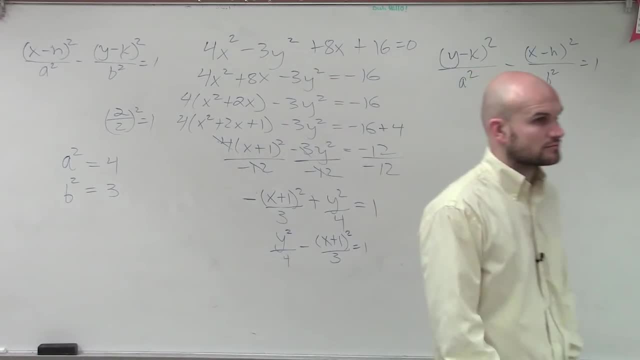 the formula that we're always going to have in this form. So in hyperbola it's not going to matter whether it's a bigger or a smaller. You're not always going to have a larger or a smaller, But I thought you said that the a squared. 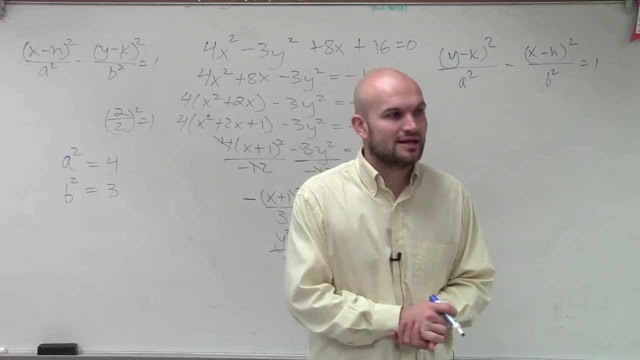 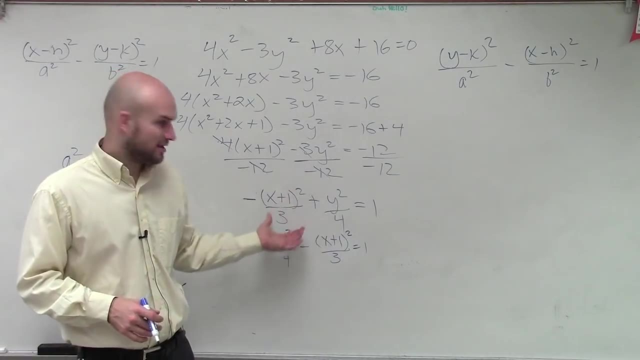 On your ellipse, on the ellipses. that's the way that you're always going to have it. Okay, You're just writing it as your subtraction, one minus the other, and then, whatever, that is what you're subtracting from. that's your a minus your b. 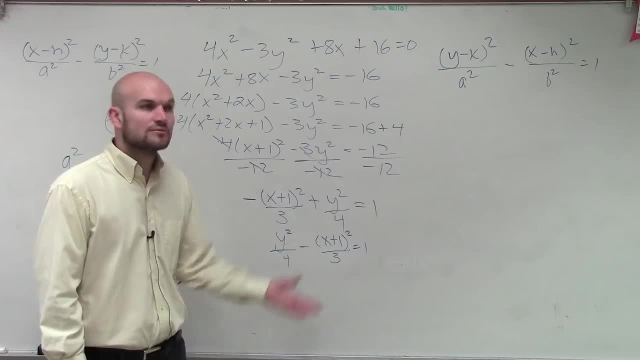 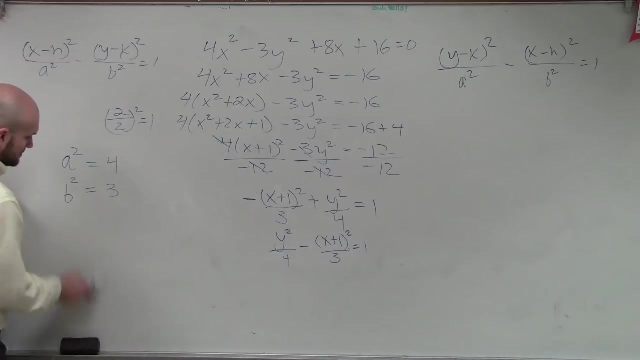 So it can be related. It can be 4 minus 5.. Yeah, That was our last example, right? So now let's go and take a look at our h and our k. So if we know our h now represents our, sorry, let's just do our center. So now, 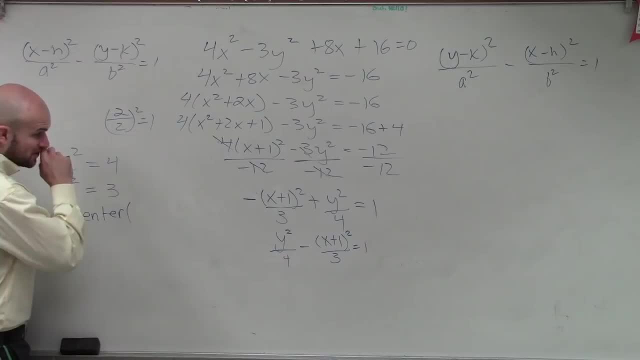 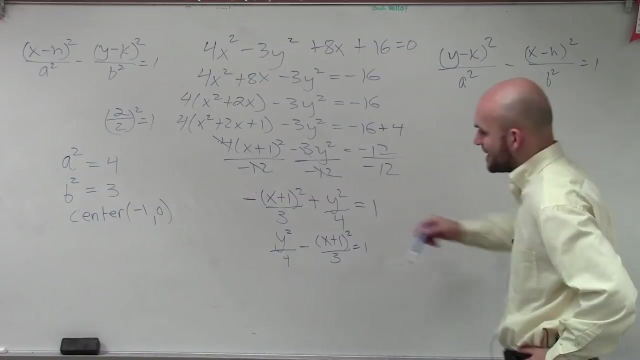 I can say the center Is going to be negative, 1 comma 0.. Yes, Yes, No, Maybe so Okay. So, ladies and gentlemen, if we have our 4 and our y, if our a squared is under our y now, this means we're going to have a vertical one, right? 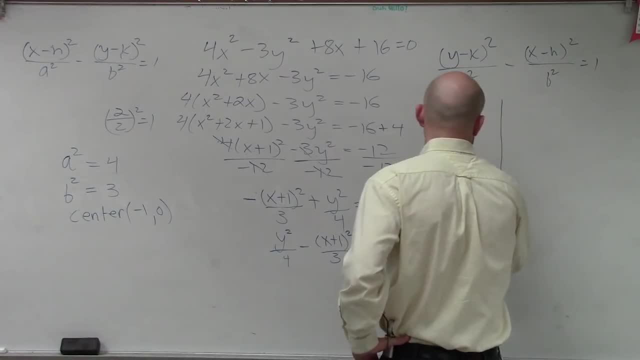 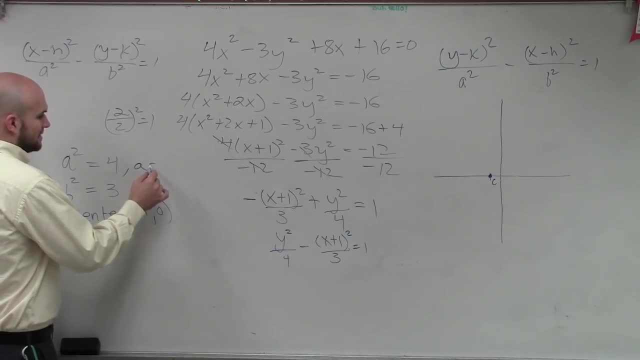 Vertical Vertical. Okay, Okay, Okay, Okay. So we know our center is at negative 1, 0.. Okay, The vertices are going to be plus or minus 4, so therefore, if a squared equals 4, we know that a equals 2.. So, to find the 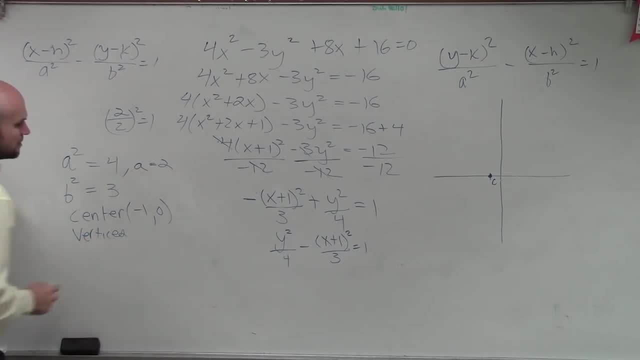 vertices. Ladies and gentlemen, are your vertices? Excuse me, pardon the interruption. Please turn your TV sets to channel 6 for the Mustang news. Since this has a vertical, Since this has a vertical transverse axis, Since this has a vertical transverse axis, our vertices are going to be on the transverse. 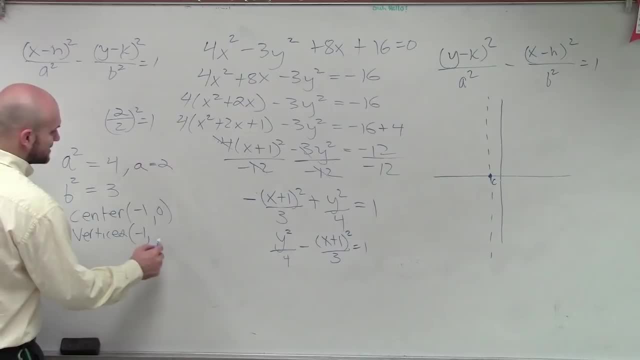 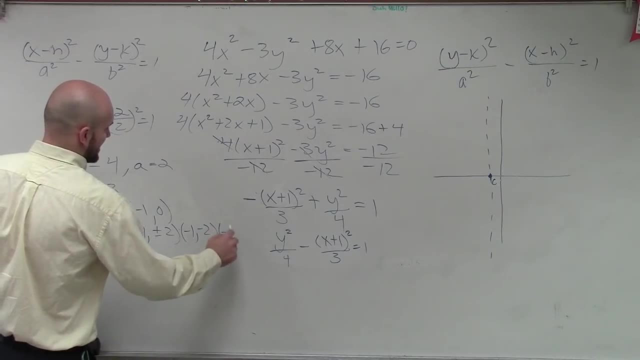 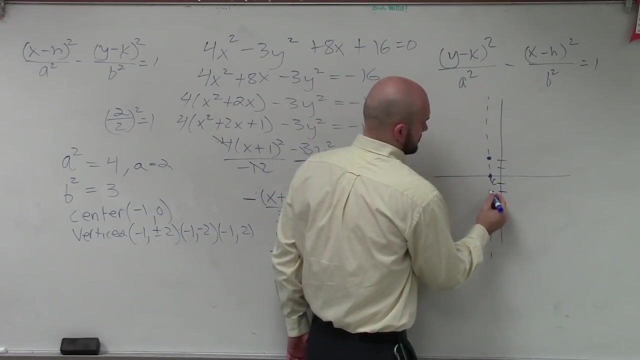 axis as well. So our vertices are going to be negative 1 comma plus or minus 2, right, Which will be negative 1 comma, negative 2 and negative 1 comma 2.. Wait, did we ever get like manuals to how to figure out the vertices, or how do you figure? 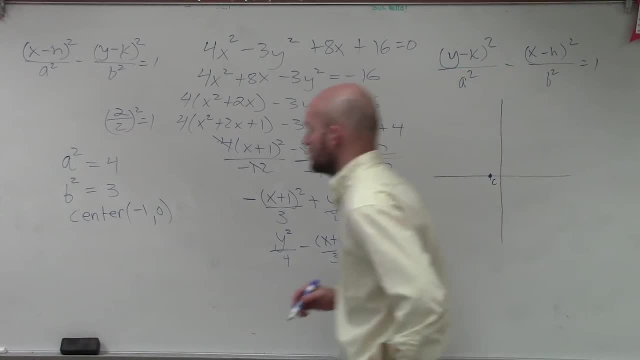 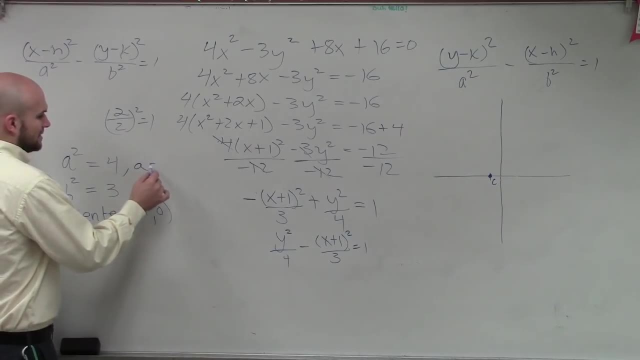 Okay, the vertices are going to be plus or minus four. So, therefore, if a squared equals four, we know that a equals two. So to find the vertices, ladies and gentlemen, are your vertices. Excuse me, pardon the interruption. 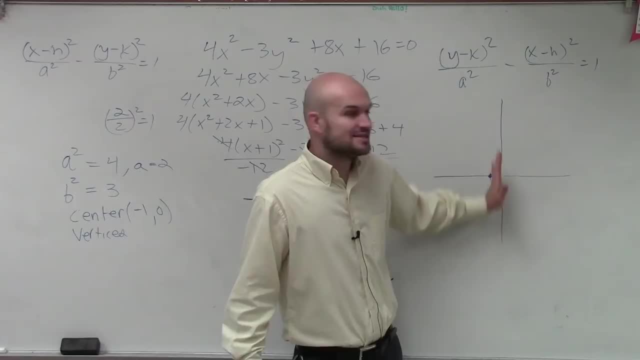 Please turn your TV sets to channel six for the Mustang news, Since this has a vertical. since this has a vertical, please turn your TV sets to channel six for the Mustang news, Since this has a vertical. since this has a vertical, you can turn your TV sets to channel six for the Mustang news. 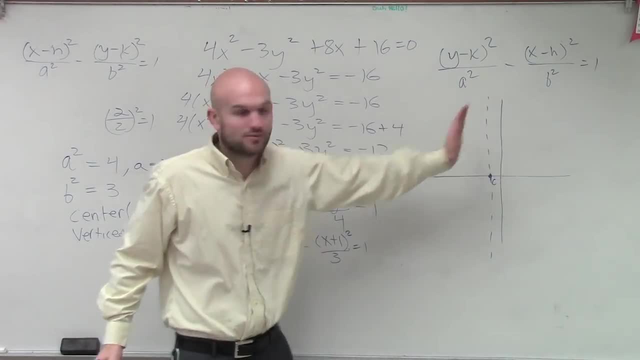 Since this has a vertical, since this has a vertical, we're going to have our vertices. but I don't know that we're going to have our vertices because you'll have to figure out how to figure out these vertices. So here are my vertices. 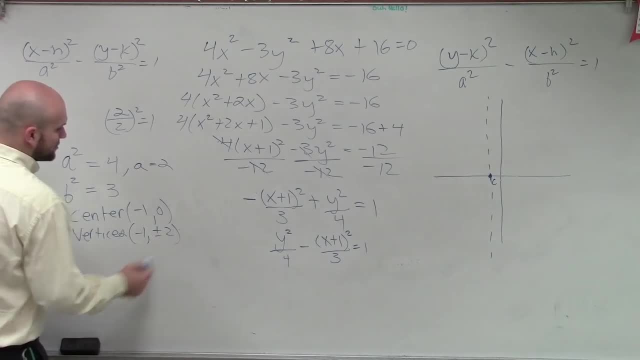 if the first one is a vertical, I wonder if this has a vertical transverse axis. our vertices are going to be on the transverse axis as well. So our vertices are going to be negative. one comma plus or minus two, all right. which will be negative, one comma, negative, two. 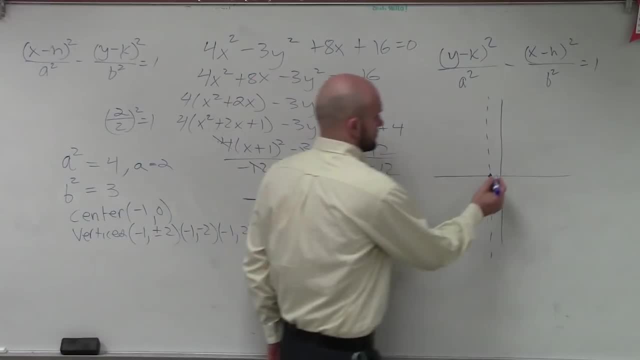 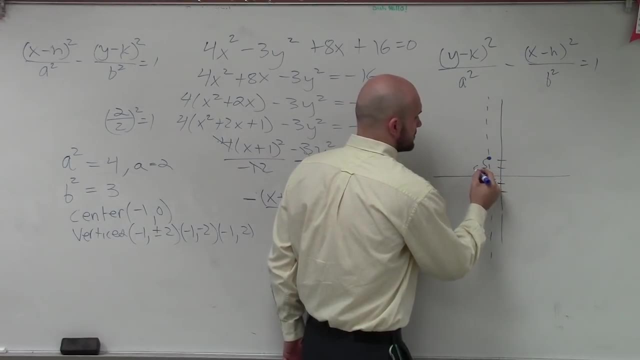 and negative one comma two. Wait, did we ever get like in the formula of just how to figure out the vertices? or how do you figure out the vertices? It's the same distance. it's a Okay, So it's the same thing as an ellipse. 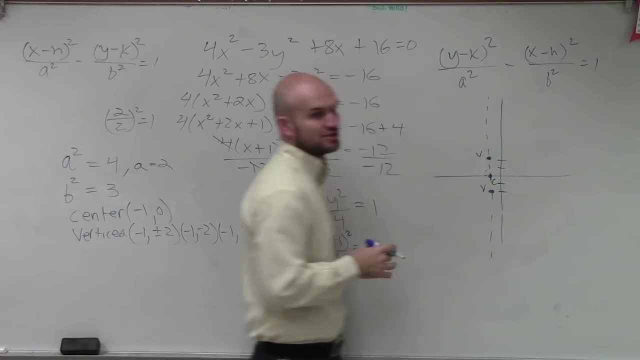 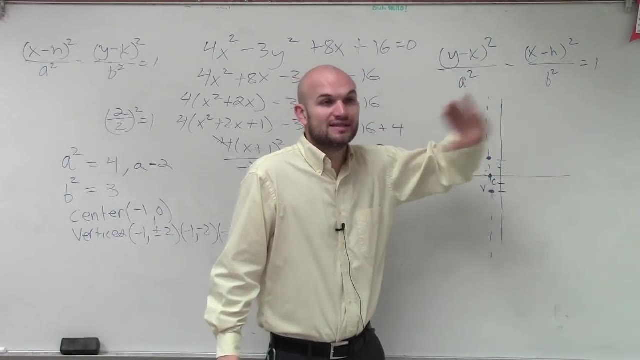 So it's the same thing as an ellipse. it's just a definition of A. The only thing you need to know is it's on the same as your transverse axis. Remember ellipses, they're all on the same major axis. well, now, they're on the same. what? 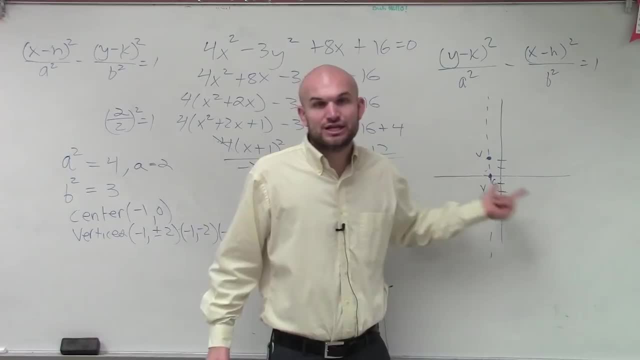 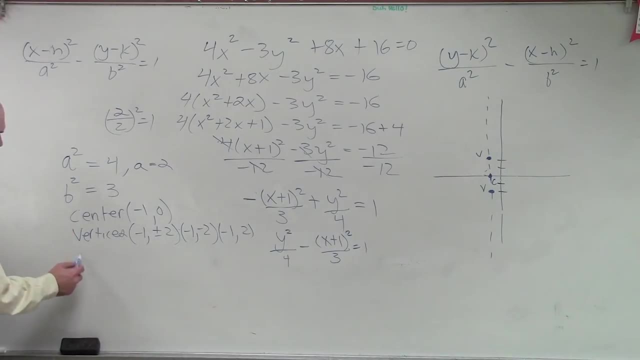 we call a transverse axis, So the H is not changing in this case because you have a vertical transverse axis. The same thing now goes with our foci. Now we need to determine what the foci is and remember the relationship we have, for 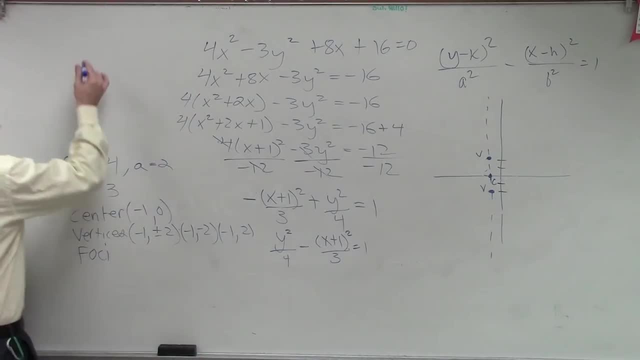 hyperbolas. Obviously, I think that was a bad reason for you to come back in class at this point in time, Because remember the definition for the foci that we had was: C squared equals A squared plus B squared. Well, we have: A squared is 4, plus B squared, which is 3.. 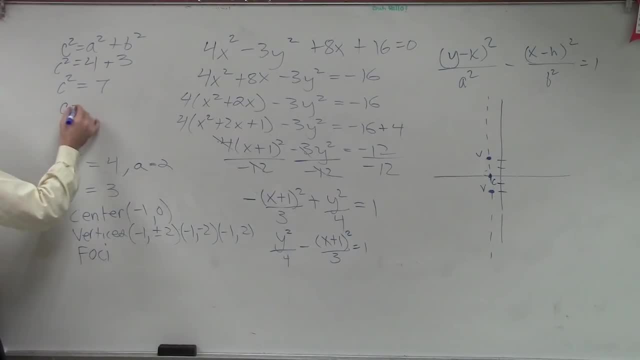 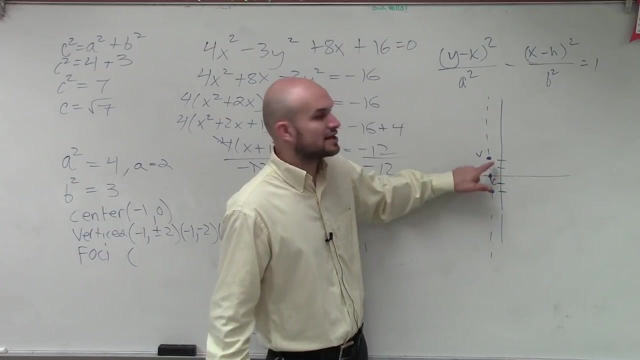 Okay, Okay, Right. You just need C squared, though, not C, right? Sorry, Do you only need C squared, not C? No, we actually need to figure out what C is, Because C is the difference. C is the distance from your center to your foci. 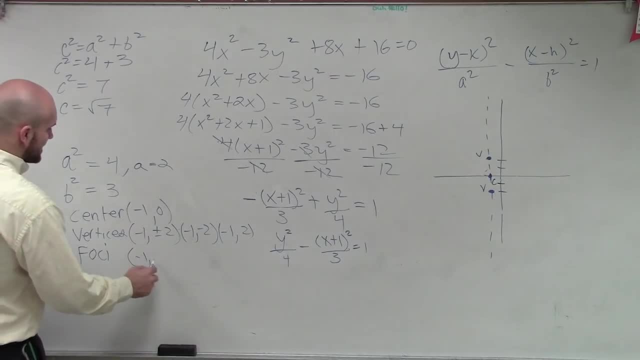 So C is the square root of 7, so our foci are going to be negative, 1 comma plus or minus the square root of 7.. Which is negative, 1 plus or, I'm sorry, negative 1 comma 0.. 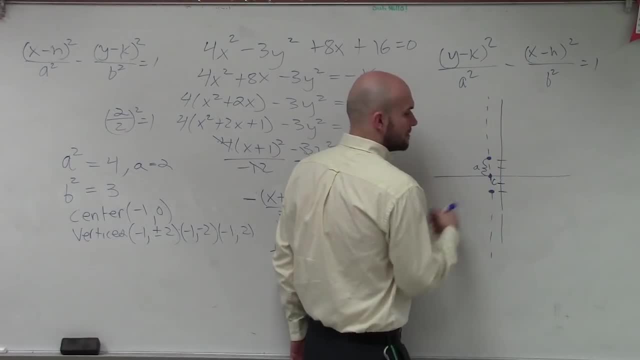 out the vertices. It's the same distance as a. Okay, So it's the same thing as an ellipse. It's just a definition of a. Okay, Okay, Okay. So it's the same thing as an ellipse. It's just a definition of a. 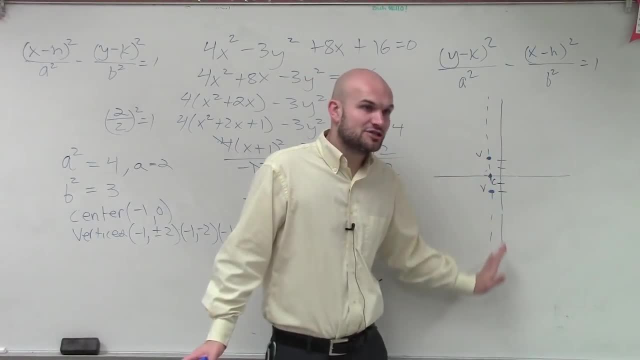 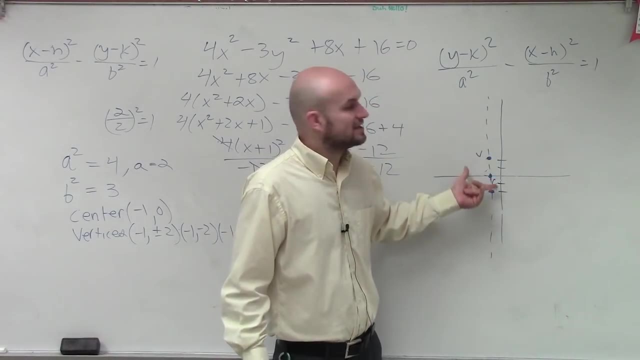 The only thing you need to know is it's on the same as your transverse axis. Remember ellipses? They're all on the same major axis. Well, now they're on the same what we call a transverse axis. So the h is not changing in this case, because you have a vertical transverse. 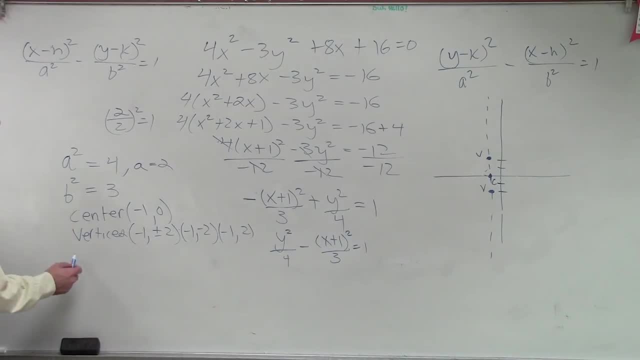 axis. The same thing now goes with our foci. Now we need to determine what the foci is And remember the relationship we have for hyperbolas. I obviously, I think that was a hyperbola. I think that was a bad reason for you to come back in class at this point in time, Because 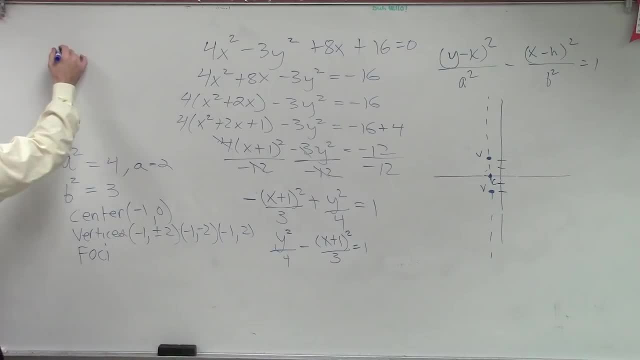 remember the definition for the foci that we had was: c squared equals a squared plus b squared. Well, we have: a squared is four plus b squared, which is three. Right, You just need c squared, though, not c, Right? 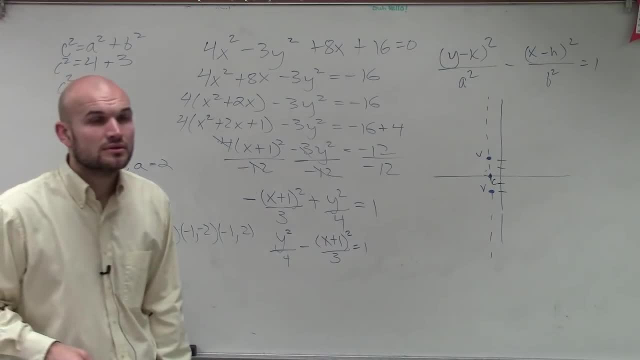 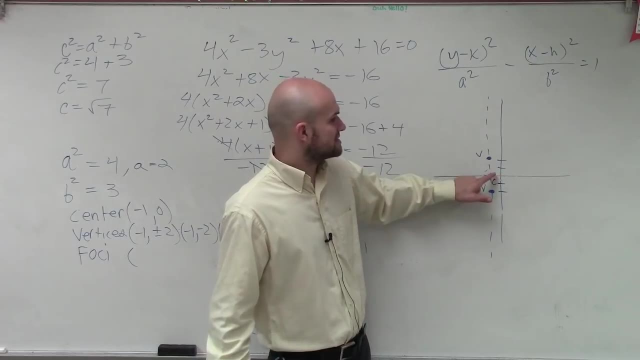 Sorry, Do you only need c squared, not c? No, we actually need to figure out what c is, Because c is the difference, c is the distance from your center to your foci. So c is the square root of seven, So our foci. 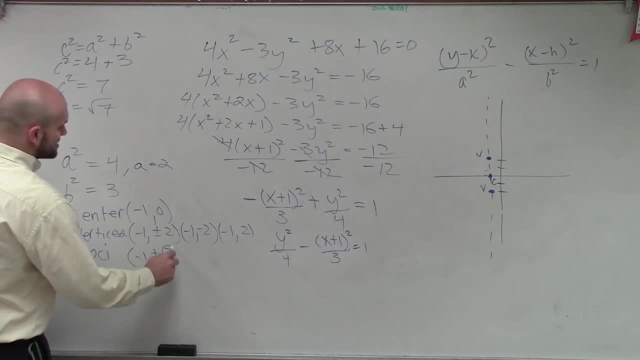 are going to be negative: one comma plus or minus the square root of seven, which is negative: one plus or, I'm sorry, negative one comma zero, sorry, zero plus or minus two. zero plus or minus the square root of seven. So 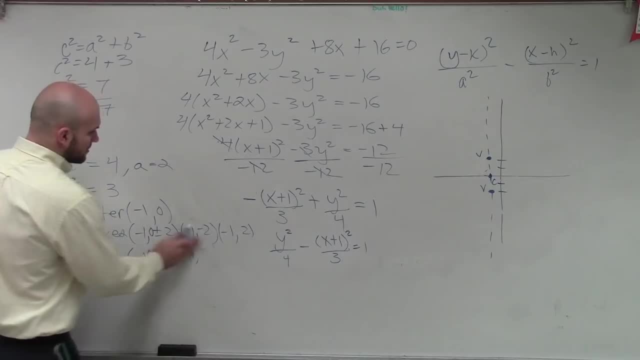 Does that matter? Yeah, why is it? Because, yeah, of course it matters. That's a huge mistake, Guys. you're taking your center and adding the vertices to your k, to the k coordinate of your vertices. This one, just. 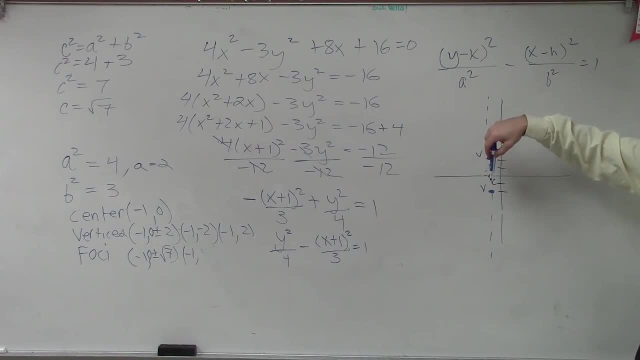 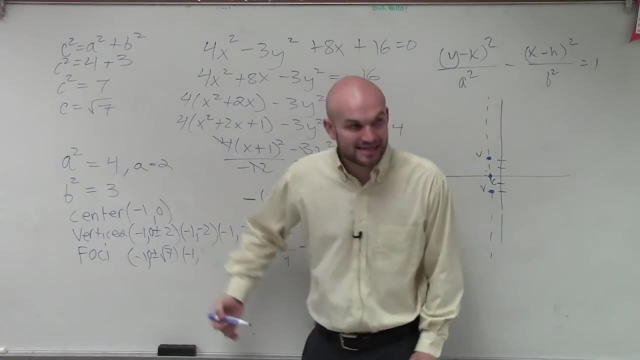 happened to be c, so it didn't matter. Yeah, but what is? what is? why do you have to put zero plus? No, you don't have to. You don't have to, and that's why I got lazy and I didn't write it. But you need to understand. 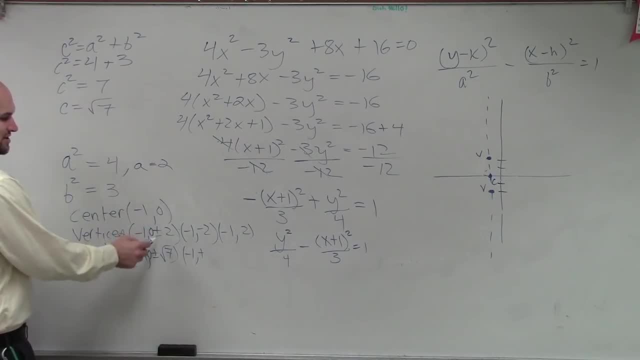 Okay, 0 plus or minus 2,, 0 plus or minus the square root of 7.. So Does that matter? Yeah, why is it? Because, yeah, of course it matters. That's a huge mistake, Guys. you're taking your center and adding the vertices to your K, to the K coordinate. 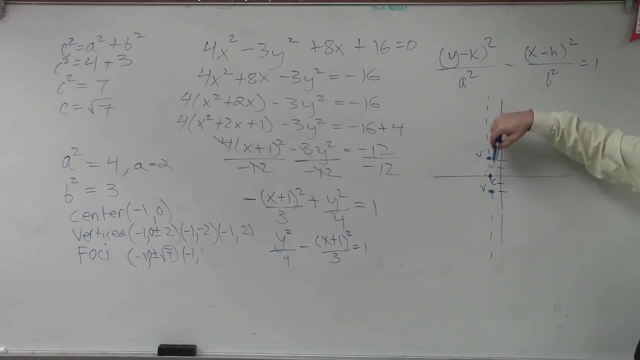 of your vertices. This one just happened to be C, so it didn't matter. Yeah, So that's why I put it in there. Why Do you have to put 0 plus? No, you don't have to, and that's why I got lazy and I didn't write it. 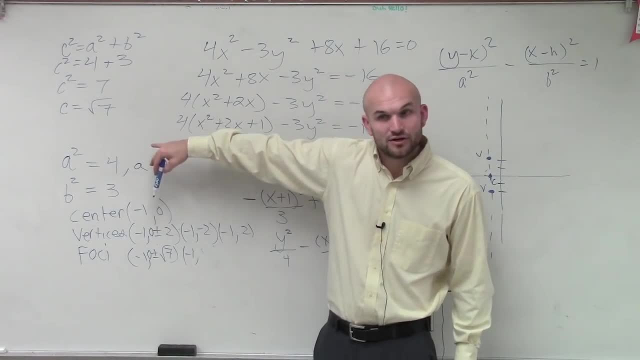 So you need to understand you're adding it to the K- K form of your center. You just need to make sure you understand that In this case, yeah, you're going to have square root of 7. And in this case you have negative 1 minus the square root of 7.. 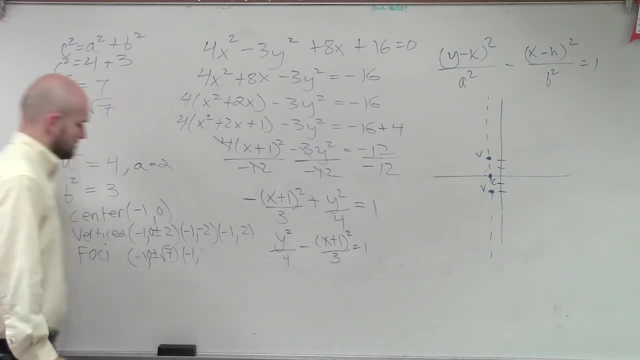 Well, guys, you can write those in your decimal form. Square root of 7 is roughly 2.6457513.. So my bottom box is the negative square root of 7.. So I'm going to write it in my decimal form. 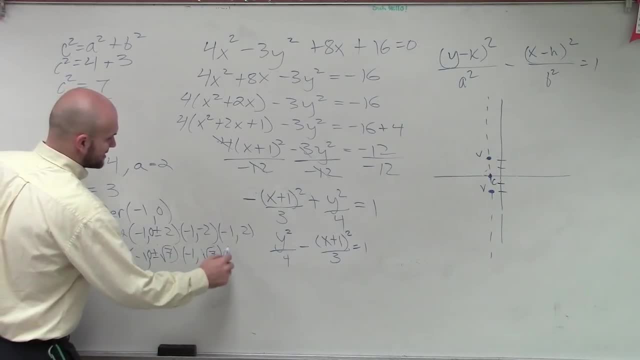 So I'm going to write it in my decimal form. So I'm going to write it in my decimal form, And then I'm going to write it in my decimal form. So I've got the square root of 7.. I'm going to write it in my decimal form. 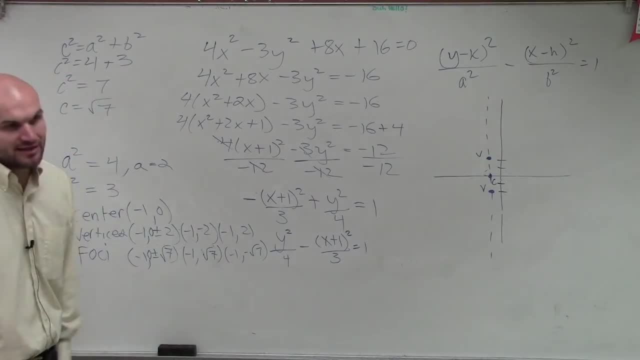 And then I'm going to write it in my decimal form. So let's go to the next one. So we have a square root of 7. And in this case you have negative 1 minus the square root of 7.. Well, guys, you can write those in your decimal form. 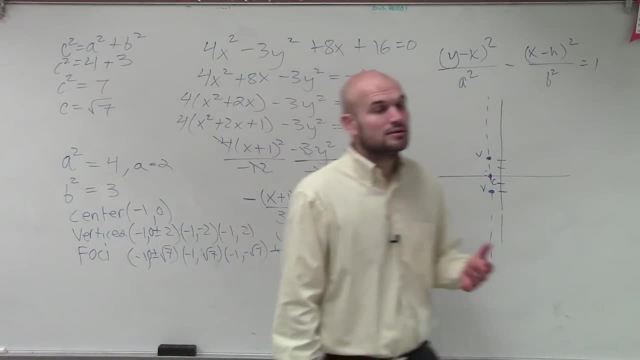 Square root of 7 is roughly 2.6457513.. I'm sorry, Say that again. Are you allowed to put negative square root of 7?? No, Because why did you not take the square root of negative 7?? But yeah, leave it in that exact answer. 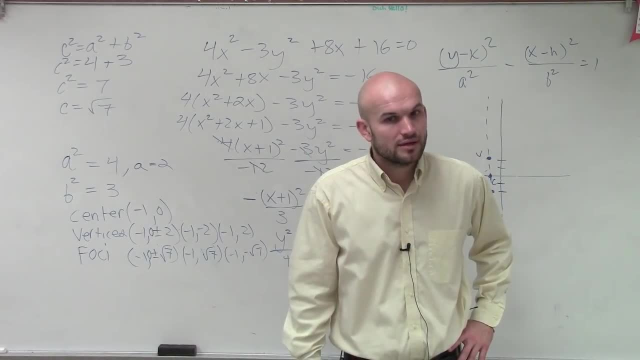 So your full side is going to be somewhere right around here, And then you'll have a square root of negative 5. And then you'll have a square root of negative 7. Because why don't you not take the square root of negative 7?? 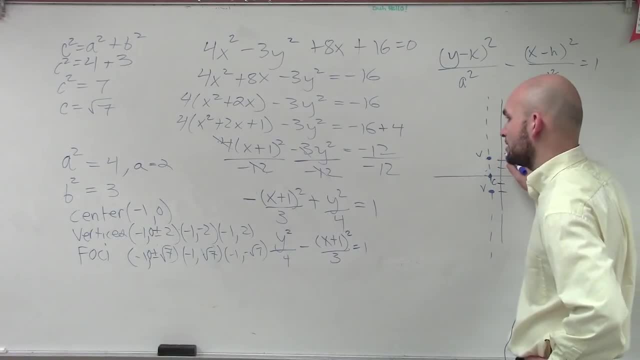 But yeah, leave it in that exact answer. So your foci are going to be somewhere right around here. Now last thing, ladies and gentlemen, remember, they're in between, They're between the center and the vertices are your foci. Now, that's an approximate value. 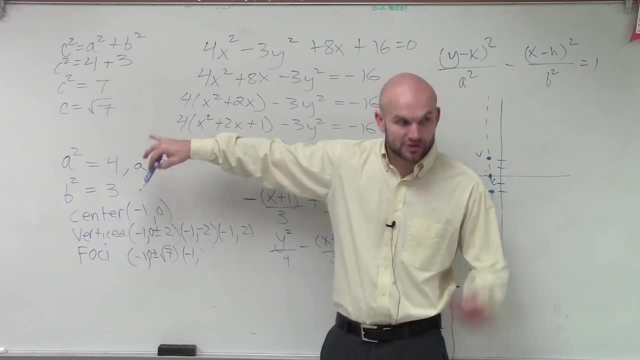 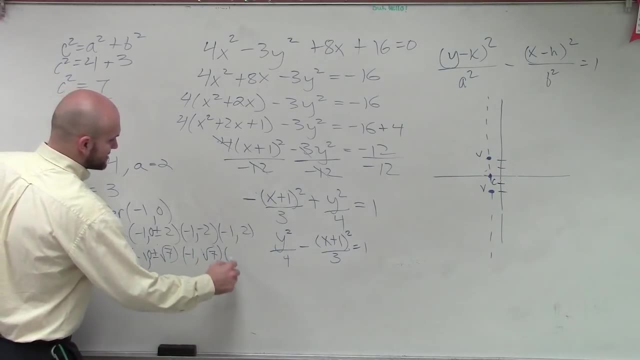 you're adding it to the k- k form of your center. You just need to make sure you understand that In this case, yeah, you're going to have square root of seven, and in this case you have negative one minus the square root of seven. Well guys, you can write those. 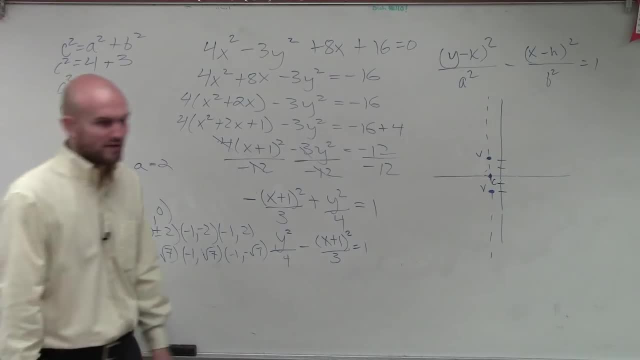 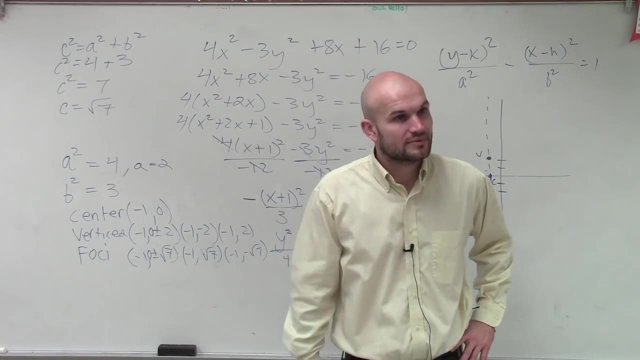 in your decimal form, Square root of seven is roughly 2.6457513.. Am I not allowed to put a negative square root of seven? I'm sorry, say that again. Are you allowed to put a negative square root of seven? 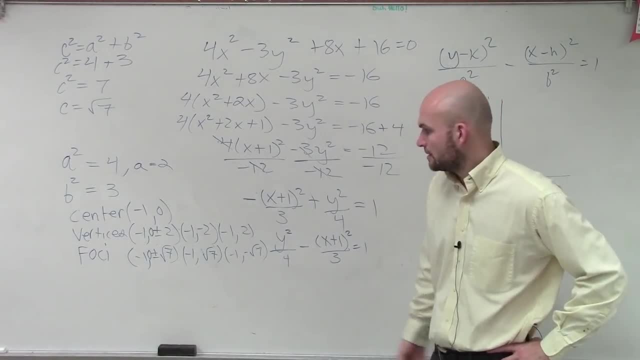 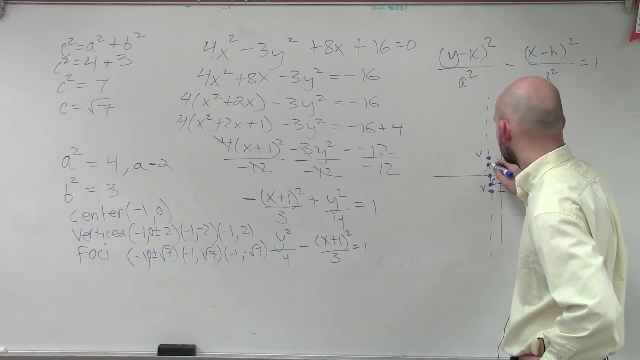 No, Because why don't you not take the square root of negative seven? But yeah, leave it in that exact answer. So your foci are going to be somewhere right around here. All right Now last thing, ladies and gentlemen, remember, they're in between, They're between. 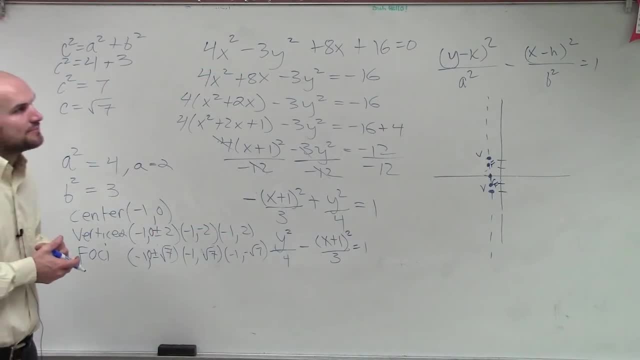 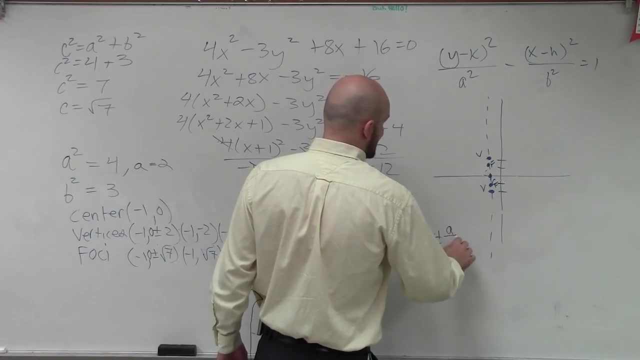 the center and the vertices are your foci Now, without that's an approximate value. The last thing, ladies and gentlemen, we're trying to do is find our asymptotes. So remember, for a vertical asymptote, For a vertical asymptote, we have: y equals k plus or minus a divided by b times x minus. 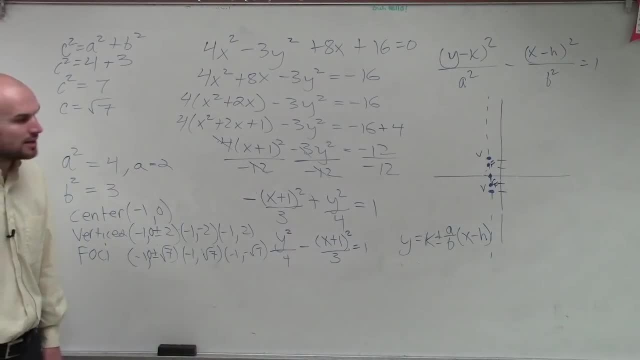 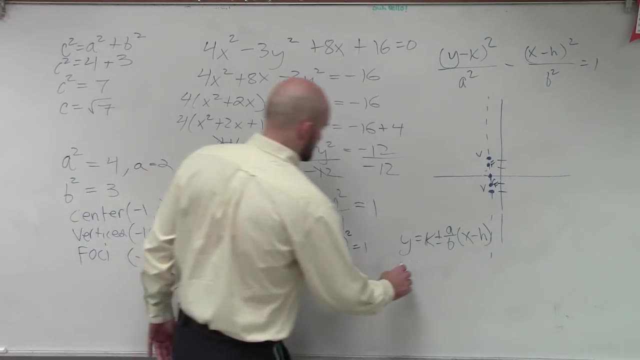 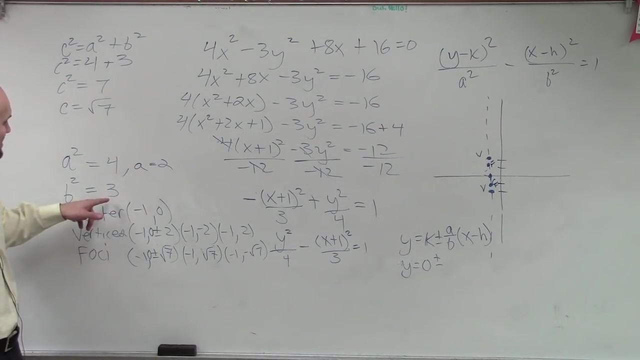 h. So all we're going to do to find our asymptotes is plug in these values. So we have our k, which is zero plus or minus a over b. So our a is two and our b is Square root of three. 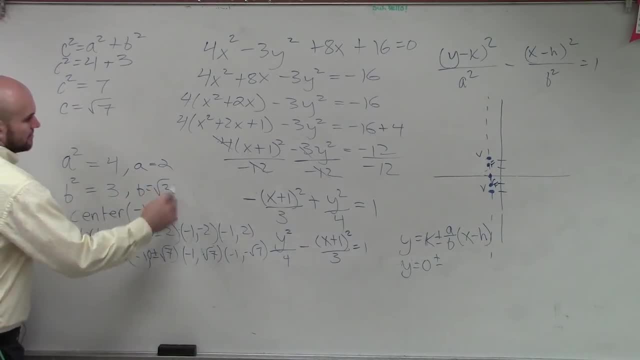 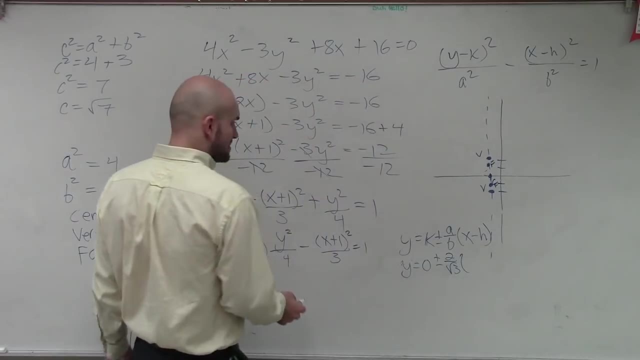 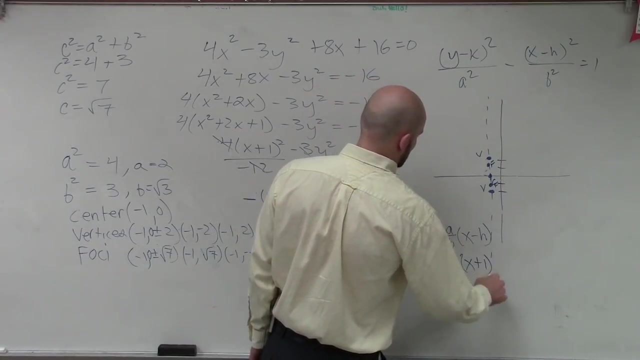 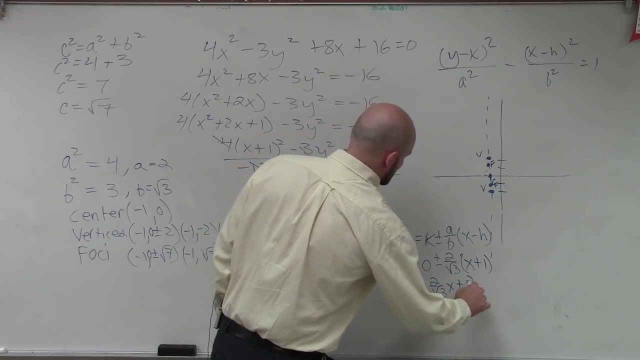 Square root of three Times x plus Times x minus h, which is negative one. You can just leave it as negative one. Oh, So then when I distribute that through, you're going to have that line. Okay, Okay, Okay. 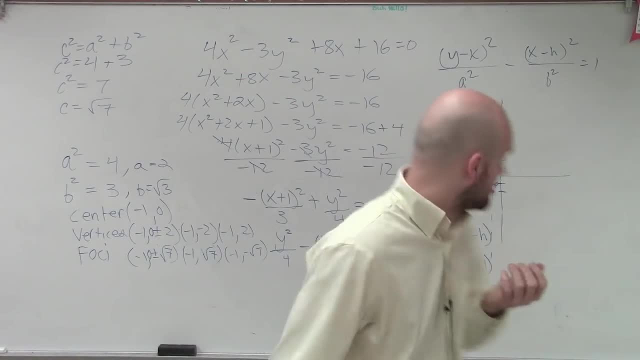 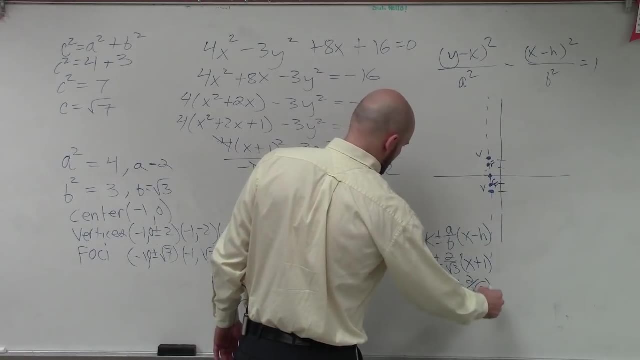 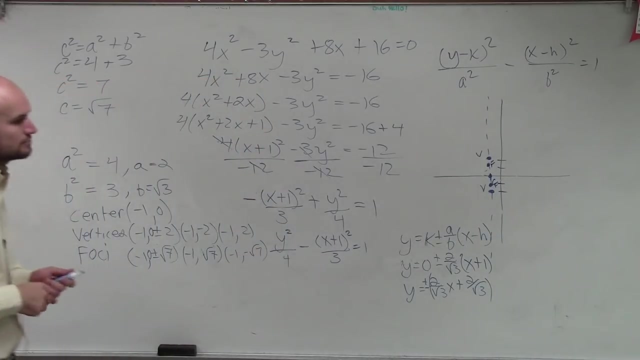 Okay, Okay. Oh, I'm sorry, It was plus or minus. Sorry, We need to do the 3.. We will learn how to graph that, but we'll practice that next class, Just so you guys understand how to find the asymptote. 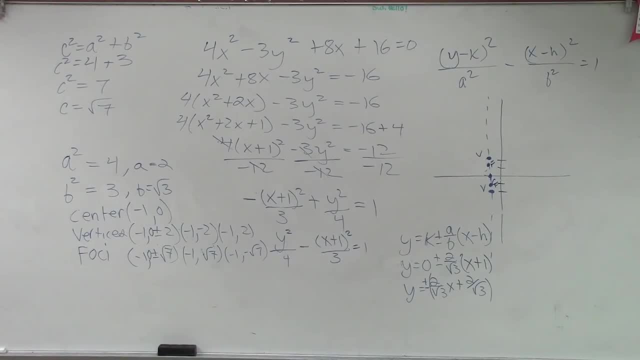 Okay, So that's all you guys are really simply doing. Let's plug it in today. 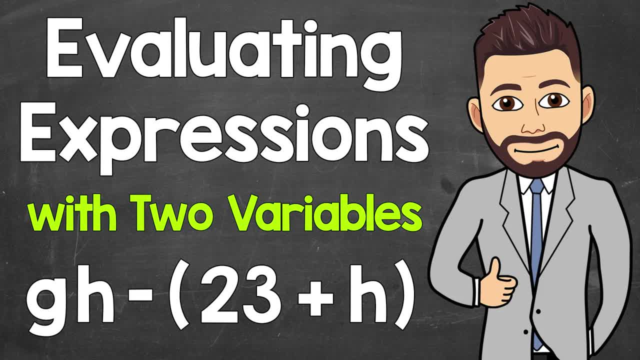 Welcome to Math with Mr J. In this video I'm going to cover how to evaluate expressions with two variables. Now, when we evaluate an expression, we find the value of the expression, so what it equals once we work through it. For our examples, we are going to evaluate: 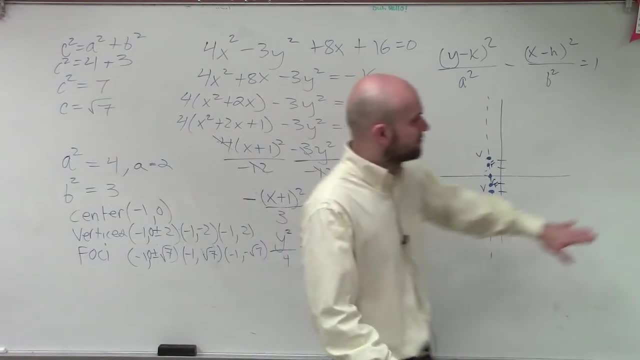 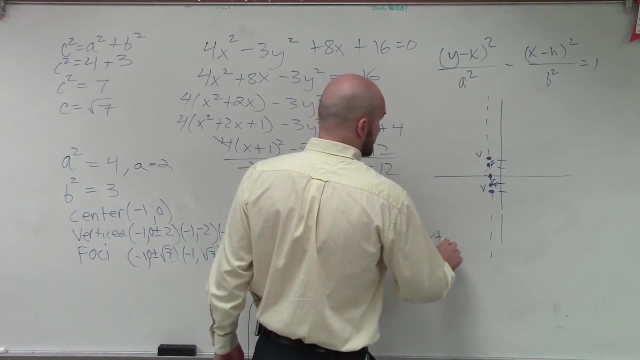 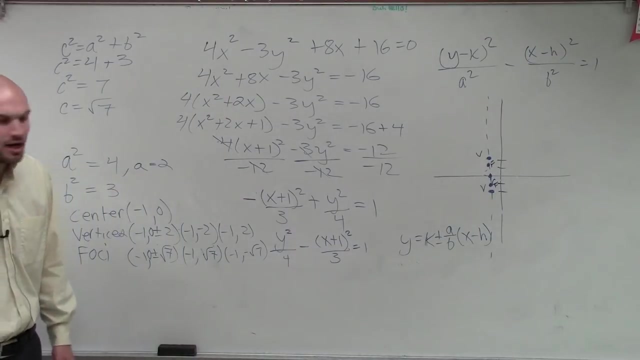 The last thing, ladies and gentlemen, we're trying to do is find our asymptotes. So remember, for a vertical asymptote, we have y equals k plus or minus a, divided by b times x minus h. So all we're going to do to find our asymptotes. 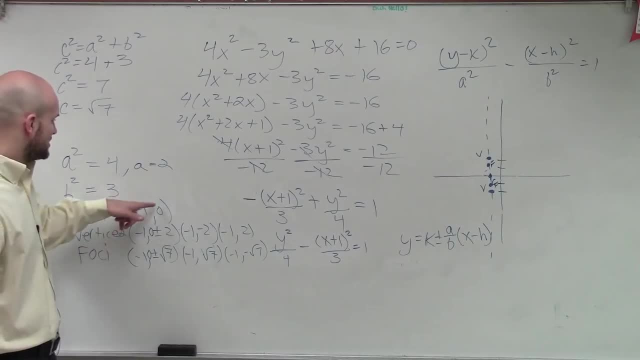 is plug in this values. So we have our k, which is 0,, plus or minus a over b, So our a is 2, and our b is square root of 3.. And so you're going to plug in our asymptotes.